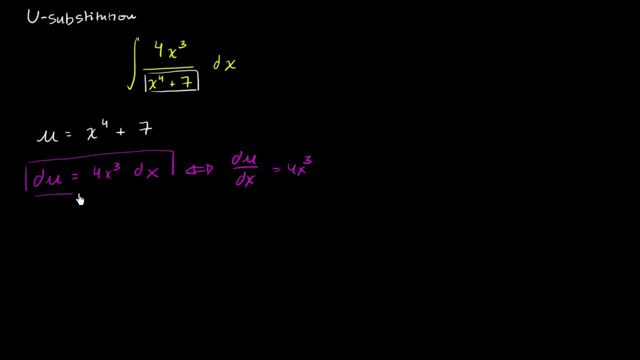 So if you wanted to go from here to there, you could kind of pretend that you're multiplying both sides by dx And we want to get it in differential form in order to do proper u substitution. And the reason why this is useful—and I'll just rewrite it up here so that it becomes pretty obvious—. 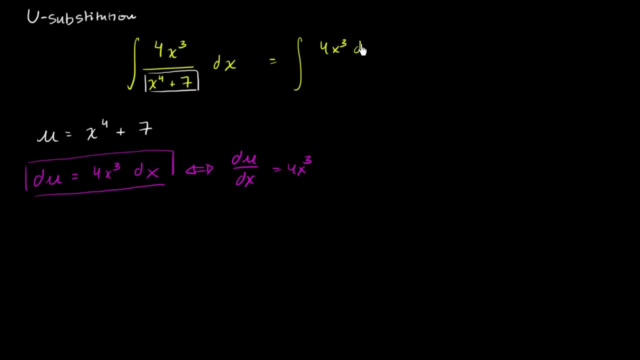 our original integral, we can rewrite as 4x to the third, dx over x to the fourth plus 7.. And then it's pretty clear what's du and what's u, u, which we set to be equal to x to the fourth plus 7.. 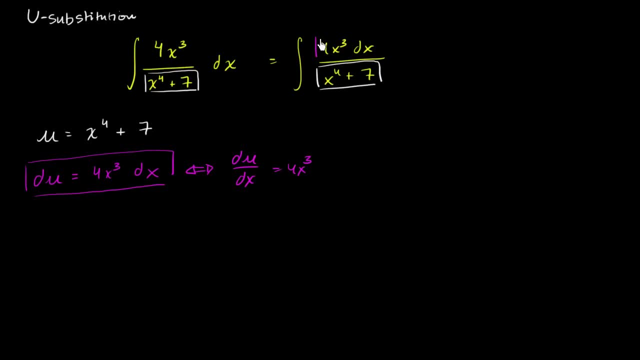 And then du is equal to this. It's equal to 4x to the third colored dx. We saw it right over here, So we can rewrite this integral and I'll try to stay consistent with the colors as the indefinite integral, what we have in magenta right over here, that's du, du, over. let's try to stay true to the colors over. x to the fourth plus seven, which is just u. 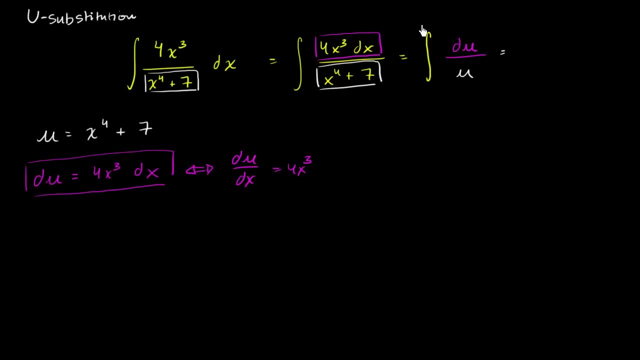 Or we could rewrite this entire thing as the integral of one over u, one over u du, One over u du. Well, what is the indefinite integral of one over u du? Well, that's just going to be equal to the natural log of the absolute value. 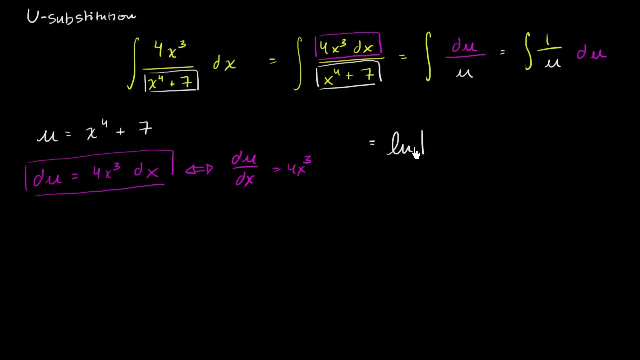 And we use the absolute value. so it'll be defined even for negative u And it actually does work out- and I'll do another video where I show you that it definitely does- The natural log of the absolute value of u, and then we might have had a constant there that was lost when we took the derivative. 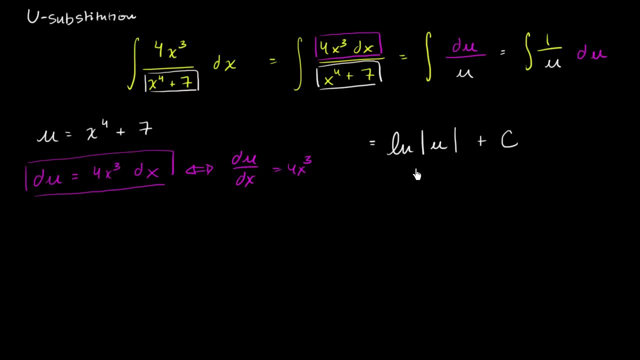 So that's what we, that's essentially our answer in terms of u, but now we need to unsubstitute the u. So what happens when we unsubstitute the u? Well then we are left with: this is going to be equal to the natural log of the absolute value of. 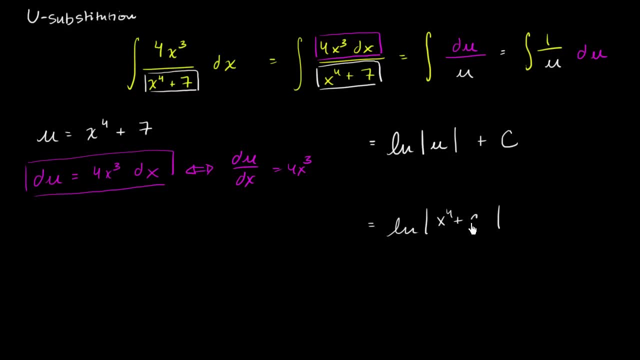 u is x to the fourth plus seven, x to the fourth plus seven, not c plus seven. And then we can't forget our plus c out here, And we are done.